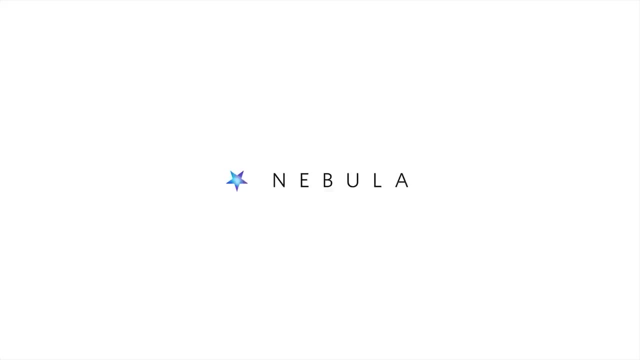 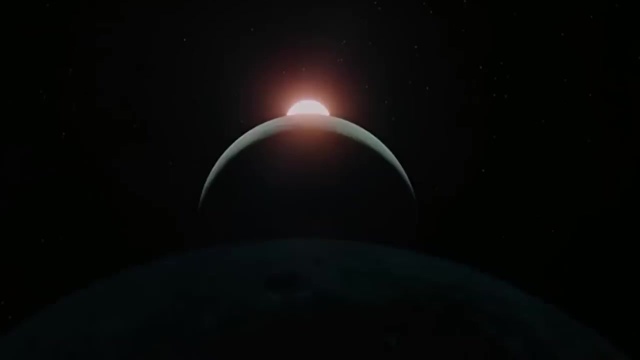 This episode is brought to you by Nebula. If you'd like to help support this channel and First Thought and the deprogram, consider signing up for Nebula at the link. below The sun, It's a big ball that can give you the power of being blind. 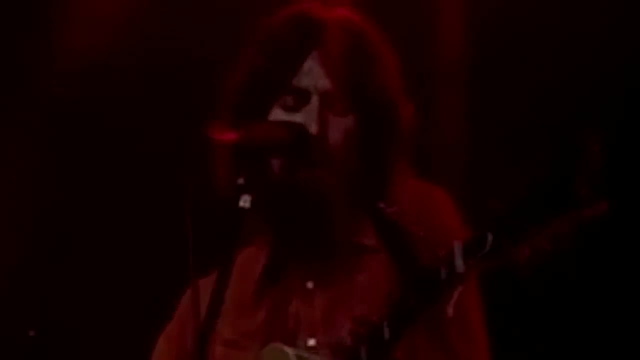 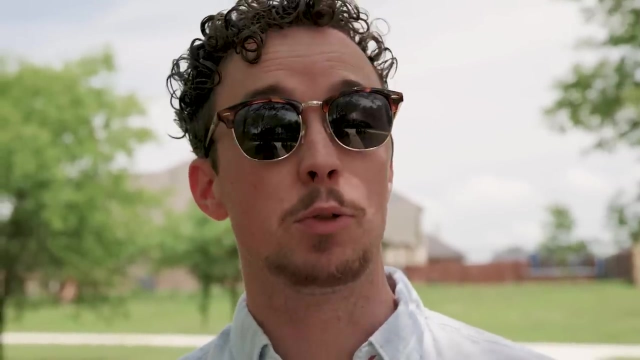 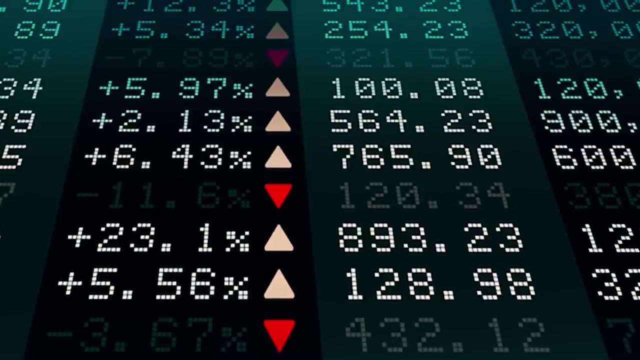 In the immortal words of the Beatles. Most people have heard of the sun As the earth's biggest and hottest ball. it's inspired countless works of art, religions and apps, But you might be surprised to find out that it's also caught the eye of countless economists, businessmen and politicians. 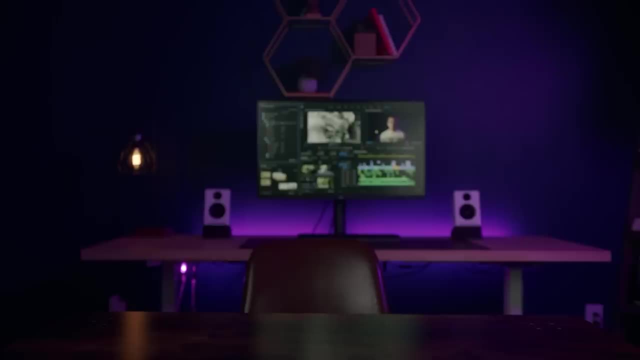 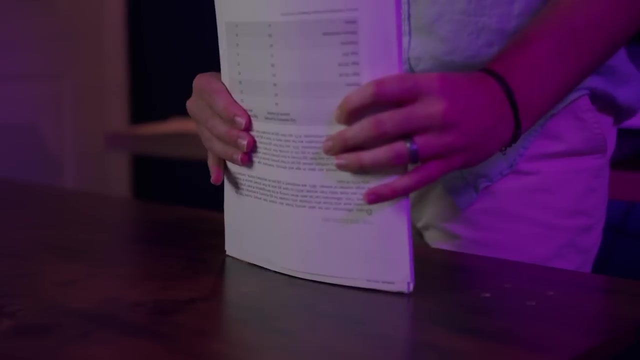 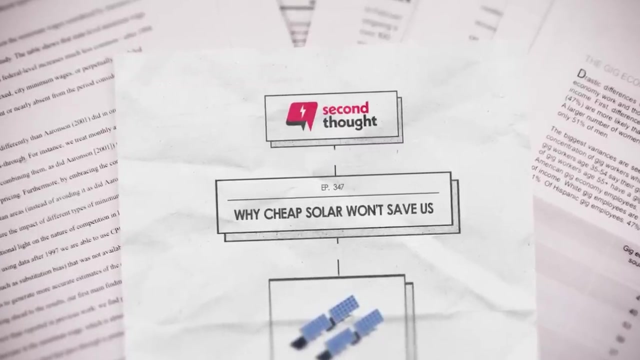 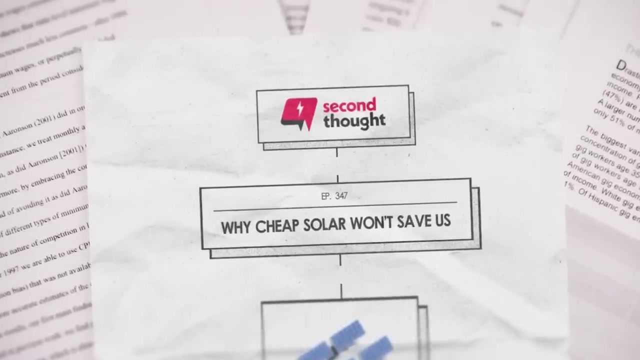 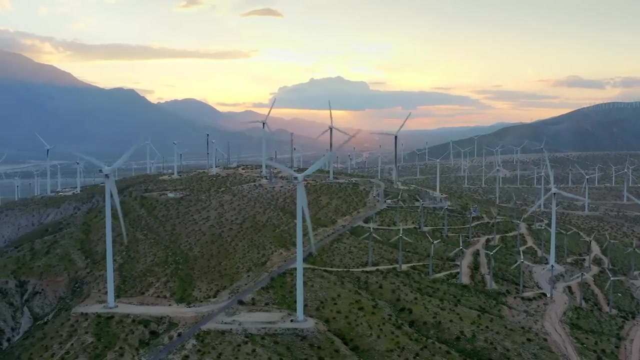 Come with me Graph time. Today we're talking about renewables, Specifically solar energy. It comes from the sky, But it's not exactly rain. It's something else entirely, An And until recently it used to be expensive. For a long time, reducing the cost of renewables has been one of the main goals of the sustainability. 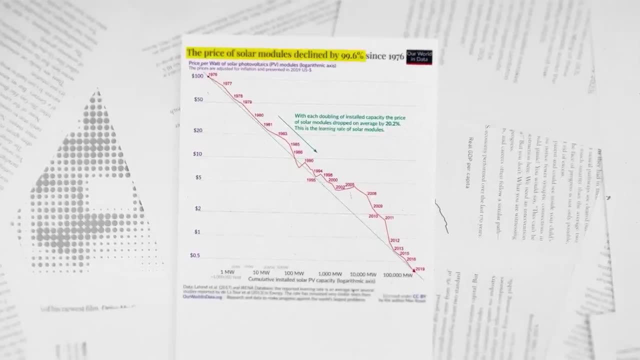 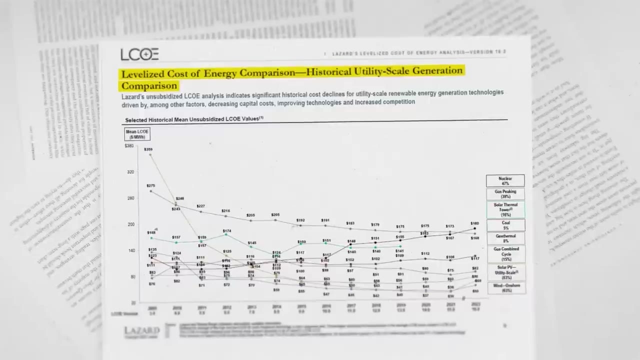 movement. And sure enough, here's the price of solar energy over the last 50 years. And now here's that same information in context. Over the past half century, solar has become cheaper than oil, gas, nuclear and even coal. And that's actually a really recent and impressive development. Coal used to be the cheapest source of energy by a lot. Even just 13 years ago, wind and solar plants were 22 and 223 percent more expensive than coal respectively. This used to be because one renewables were an emerging, small-scale and therefore costly. technology to both develop and implement. And two, it came with a high upfront investment cost that takes a long time to generate an appropriate return. Think building a whole new solar farm or a field of windmills from scratch. Banks considered them a high-risk investment at that time. 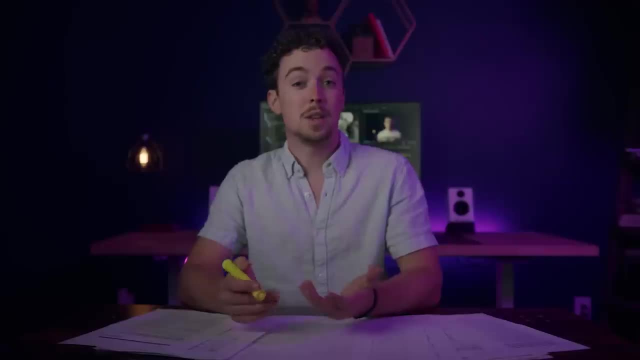 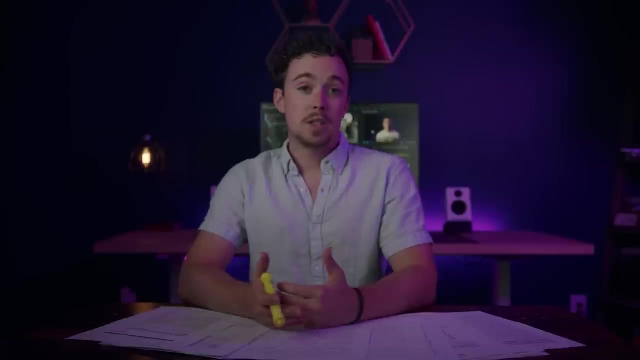 And generally didn't want to put money into renewables, Something that they, frankly, didn't even care to consider, given the enormous amounts of subsidies going to fossil fuels and how profitable that makes them. In the face of this lack of investment, governments had to step in. 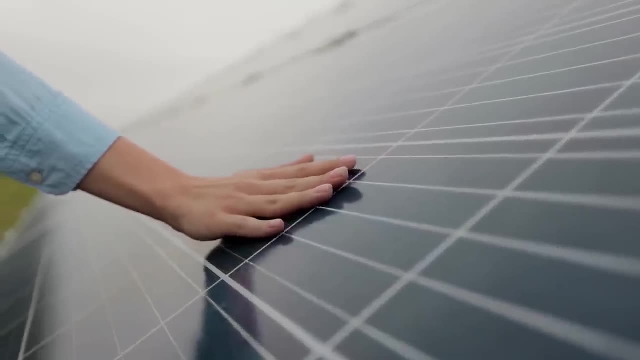 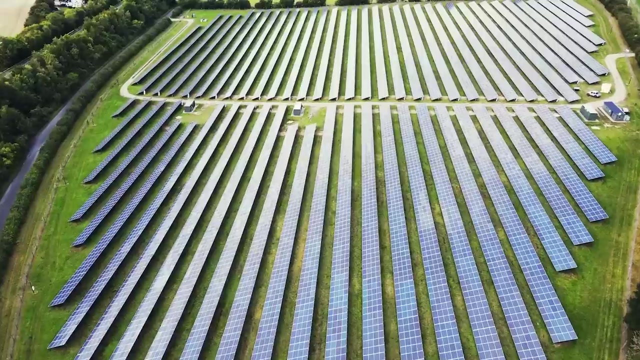 Through a combination of continuous improvements in the technology's efficiency. subsidies slash market interventions by governments, notably in Germany, and a massive production effort in China, generating economies of scale. solar's price per megawatt-hour went down almost 90 percent just between 2009 and 2019.. 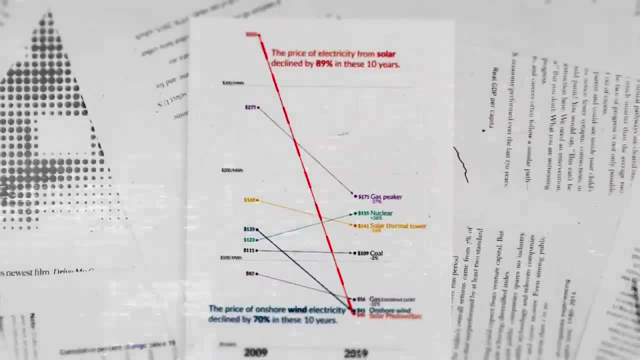 And that's not all. In the last decade, solar's price per megawatt-hour went down from $1.5 billion to $1.5 billion in 2019.. Essentially, doing in 10 years what NFTs managed to achieve in the 12 months of 2021.. 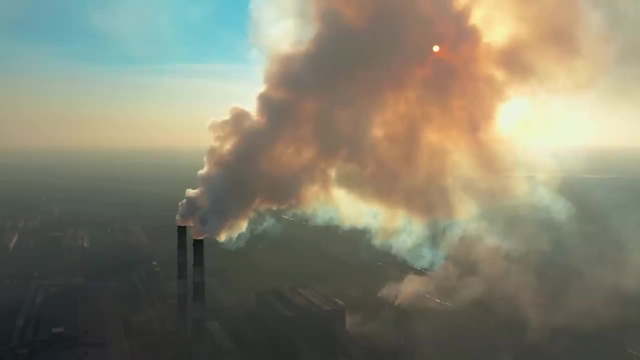 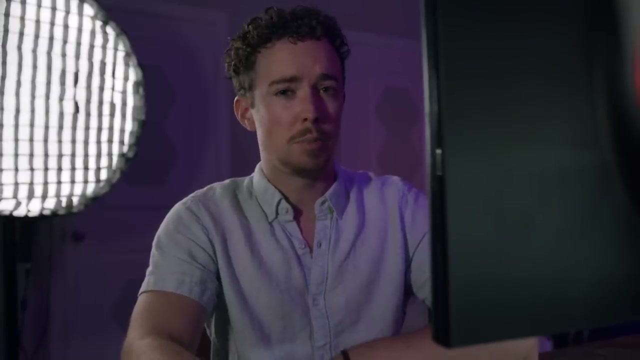 That's what's in the eye-opening chapter of every econ book you'll read in college And as far as climate change goes, that sounds like the problem should solve itself. If people do what people do and just follow the bargain, the cheaper and, coincidentally, 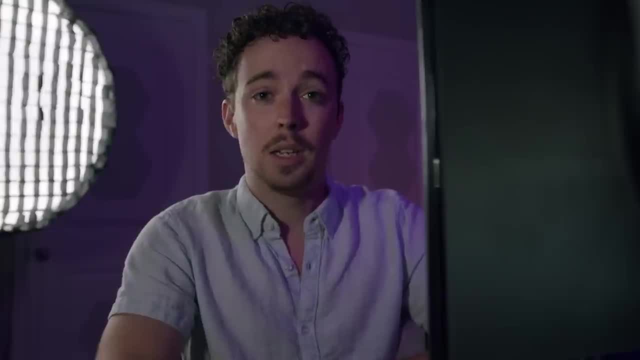 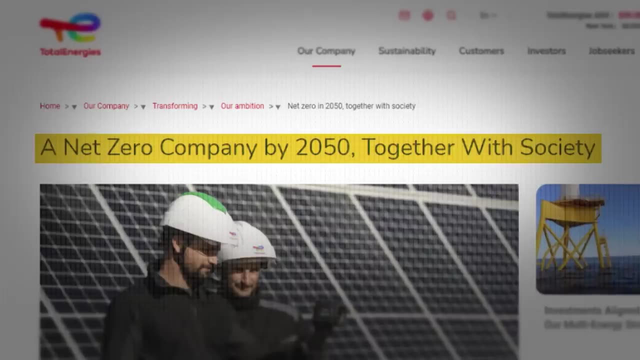 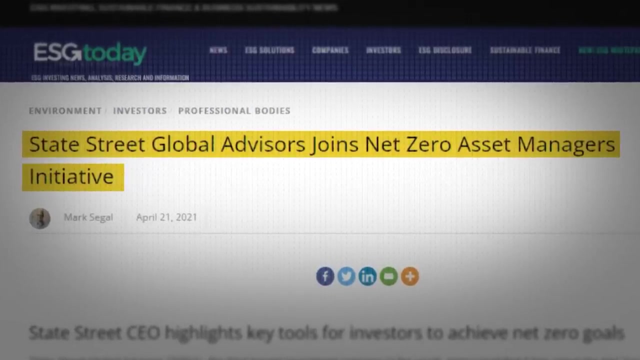 more sustainable energy should take over And, seemingly in line with that positive prediction, basically every major company, even in the fossil fuel industry, from BP, Shell and Total through massive investment firms like BlackRock and State Street, have made pledges to reduce carbon emissions and invest in renewables. 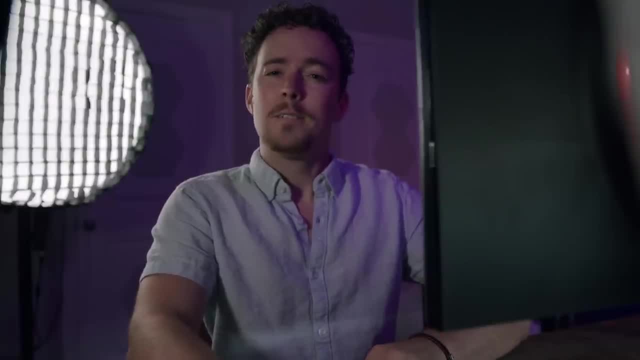 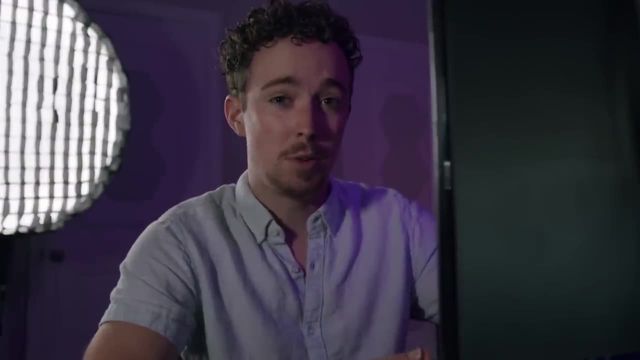 Now that renewables are so cheap, it really feels like we're good to go. But we're probably not, And I know you think you know why And you're wrong. You're expecting me to use the rest of this video to talk about the various problems. 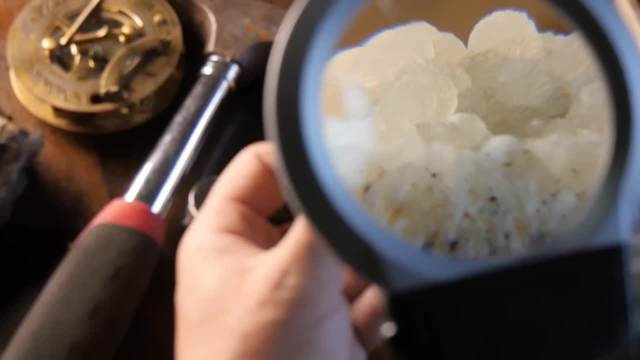 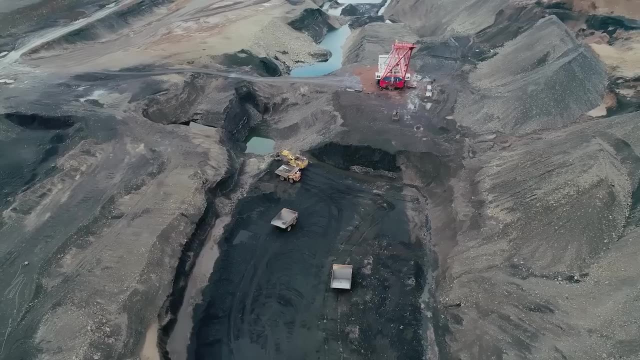 with solar energy, The non-renewable rare earth minerals it requires, The horrible conditions of exploitation that are used to extract them and the neocolonial trade relationships that this generates, Or something like the pollution solar panel production generates and the difficulties in recycling them. 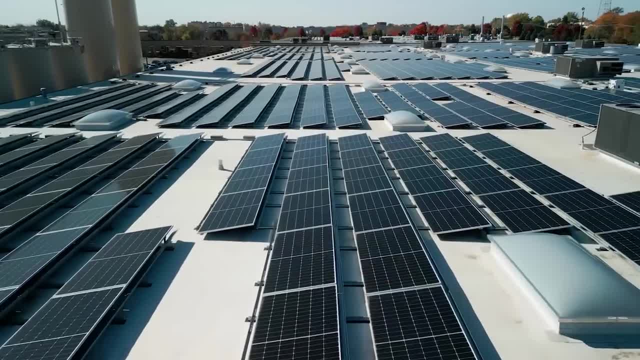 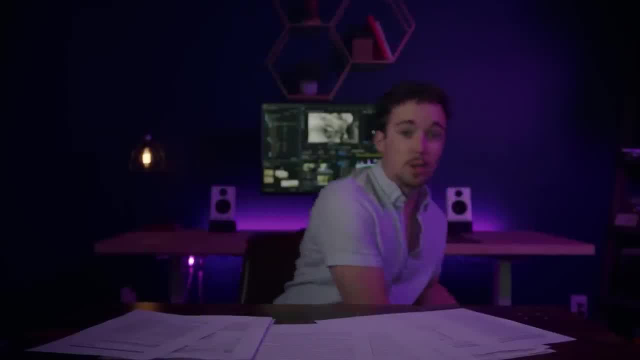 Or maybe you're thinking of the problem of energy storage and day-to-day reliability we often hear about in the case against solar. But you're dumb, I'm going to blow your tiny little pea brain to smithereens Because I'm putting all these problems in our get back to it later- box. 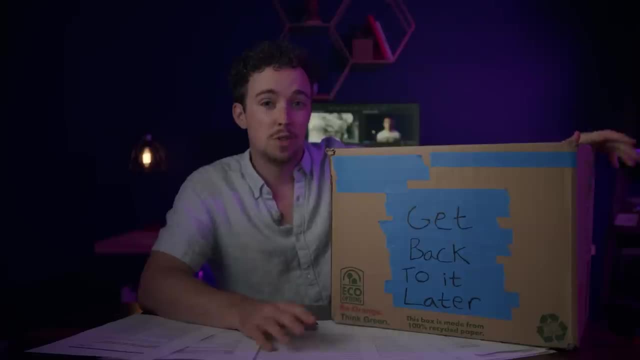 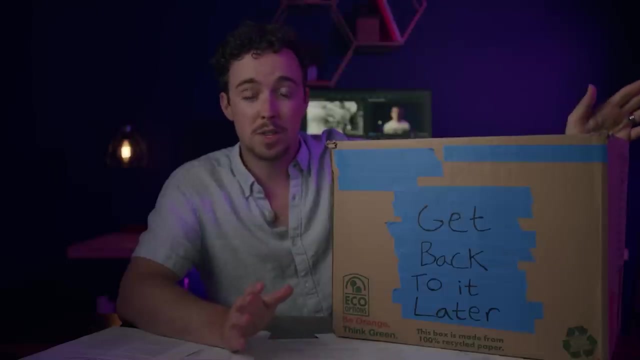 This video is about something else. The thing is that, even if we assumed solar energy could be a silver bullet solution to climate change, instead of looking at a more comprehensive approach, if we could set all these problems aside, there's still something that's been plaguing the renewable energy. 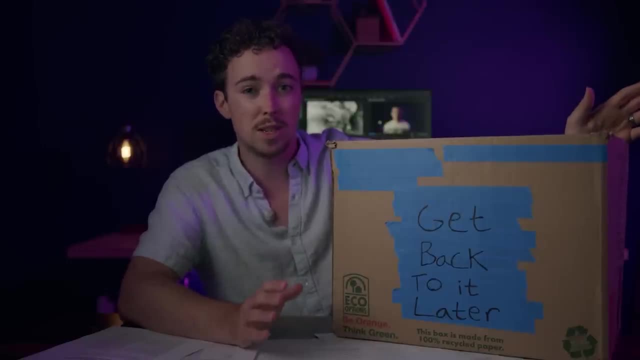 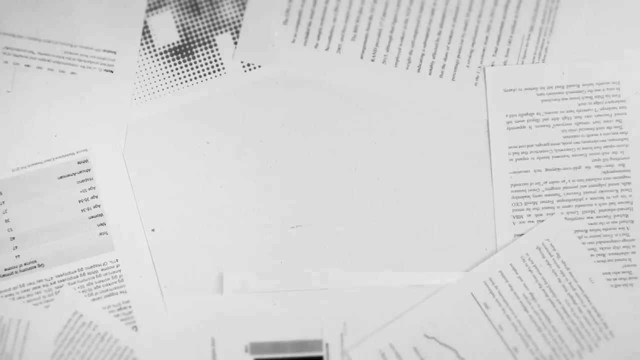 transition this whole time that low prices don't fix and might actually even hurt. They may be cheap, but renewables just aren't profitable. In May 2019, the International Energy Agency found that, for the first time since the 2000s, 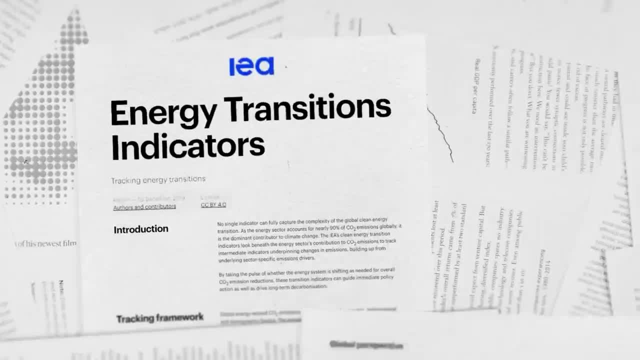 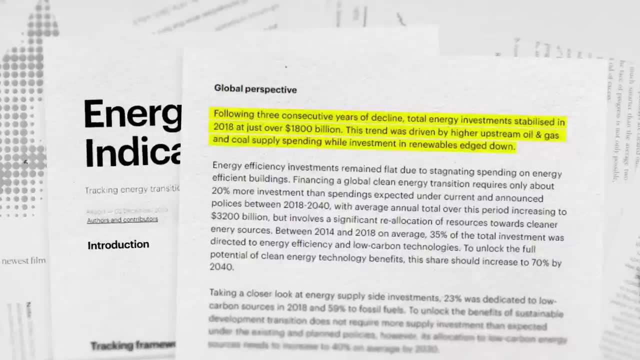 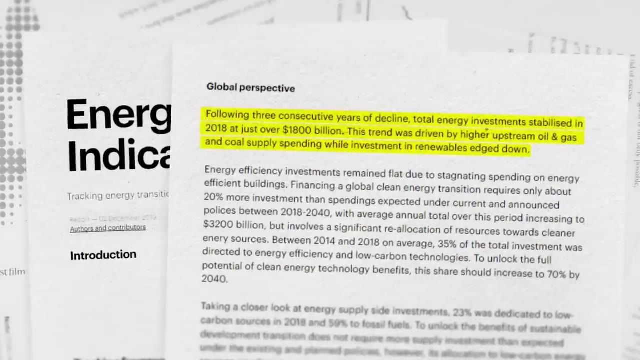 renewable energy deployments started stagnating For three years. that same agency had already found that investment in renewables was on the decline. Less money going in, fewer projects going out, despite nearly a decade of prices going down and governmental measures specifically designed to spur action. 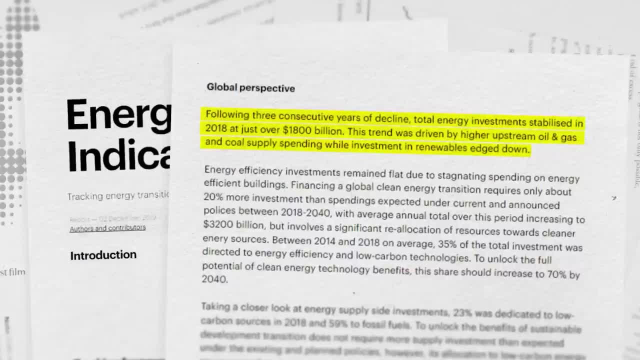 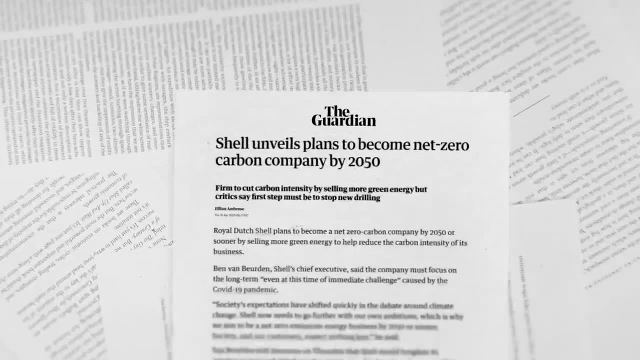 Prices had quite simply never been lower, but investment and deployment weren't following through like the conventional economic cycle. In fact, this is what the economic story of Cheaper Product Wins predicts. But this is still around the same time that the fossil fuel giants like Shell were announcing 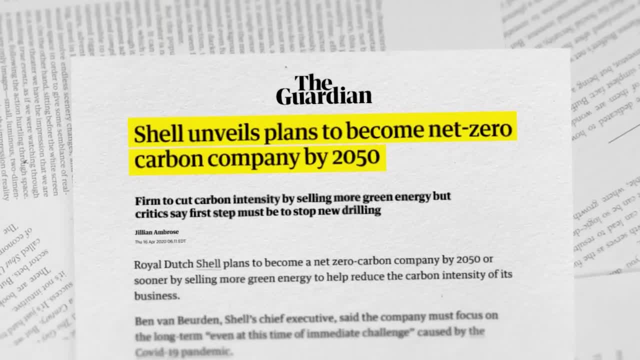 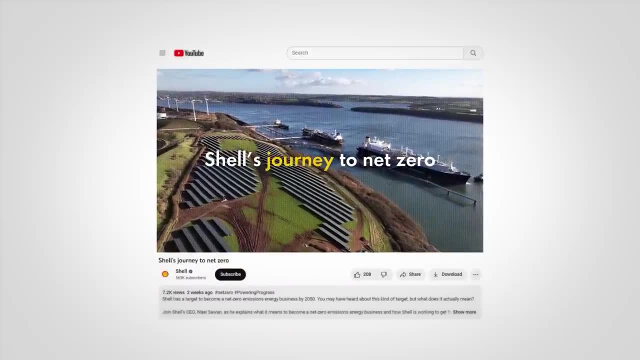 to the public their net zero goal for 2050, which they said would be coming from a massive upscaling in renewables. But look beyond the flashy headlines and these stats about declining investment and deployment start making more sense. Shell was actually a lot less committed to the renewable transition than they wanted. 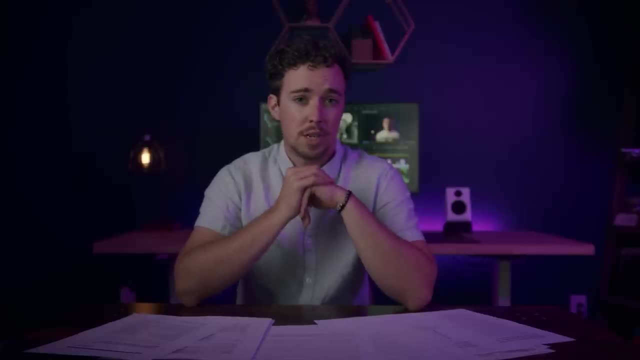 to make it seem What looked like bold, definitive statements of sustainability were not. They were more about the cost. They were about the cost of the industry. They were about the cost of the society. They were about the cost of the economy. 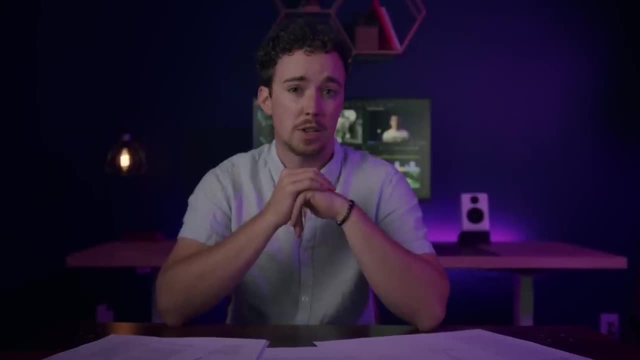 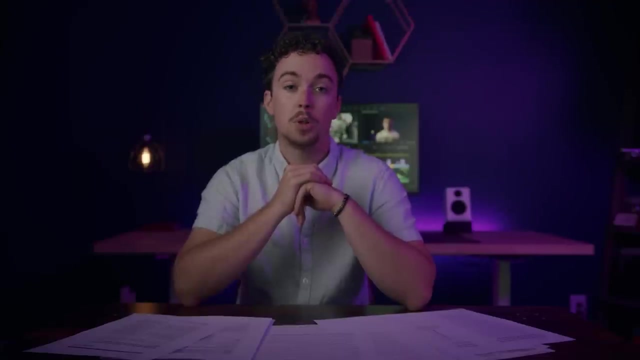 And the last two statements that were most likely to be held in the press were actually tepid, conditional half-promises that didn't commit Shell to any sustainable action whatsoever And highlighted what matters most when private enterprise looks to invest in renewables. Specifically, Shell put three conditions on its transition to renewables. 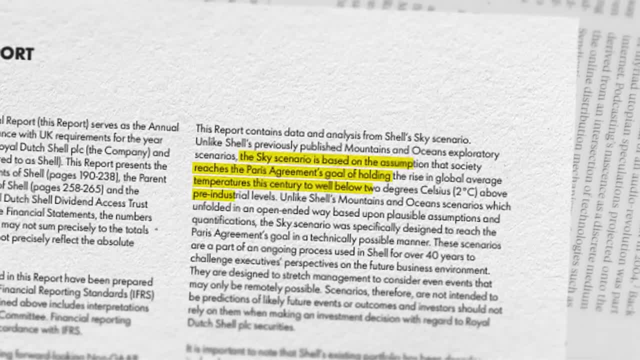 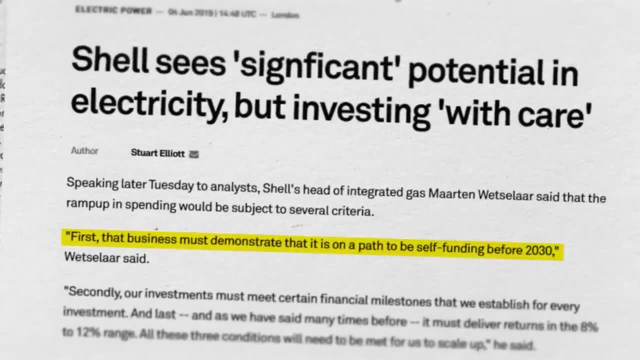 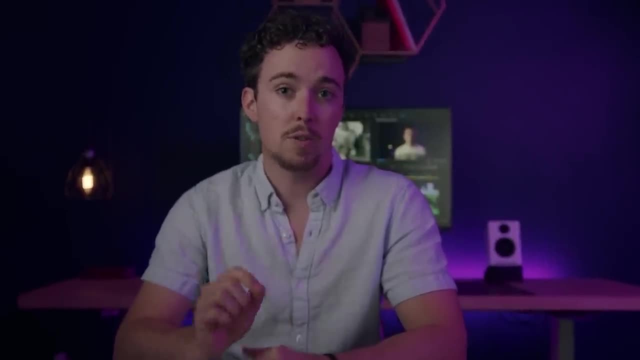 1. That the society- a term that is very much not defined- would follow through on the Paris agreements. 2. That this venture would be- quote- self-funded And, most importantly, 3.. 2. invest substantially in renewables if, and only if, it delivers the appropriate profits. 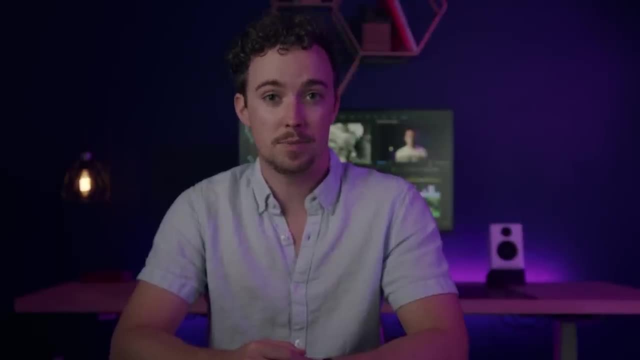 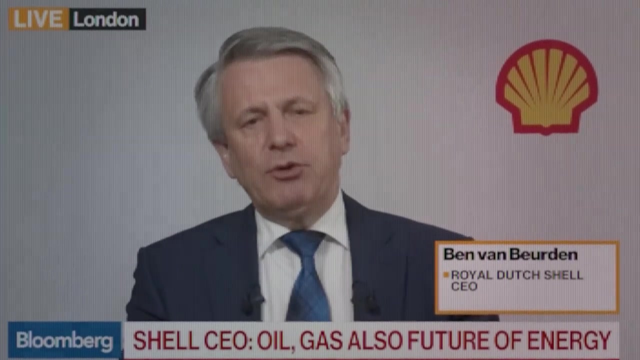 which, for Shell, means an 8-12% return on investment. Now, that is a business of the future, a business that doesn't really exist at this point in time. so that's why we want to move cautiously and we will only ramp up this business as we see these proof points of an 8-12% return come through. That last condition is the most important one you need to remember. The first two are other ways for Shell to bail out clauses that basically amount to little more than promising to jump if they get pushed out of the plane. 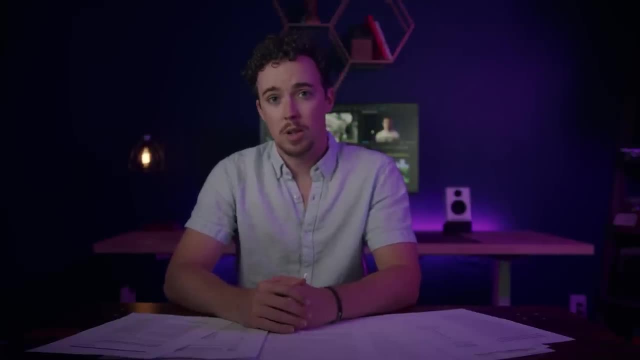 But that last condition, profitability, is the most crucial. Shell- and this goes for basically every other fossil fuel company that's come out with a net zero promise- places its renewable transition on the condition of a high, in this case 8-12%. 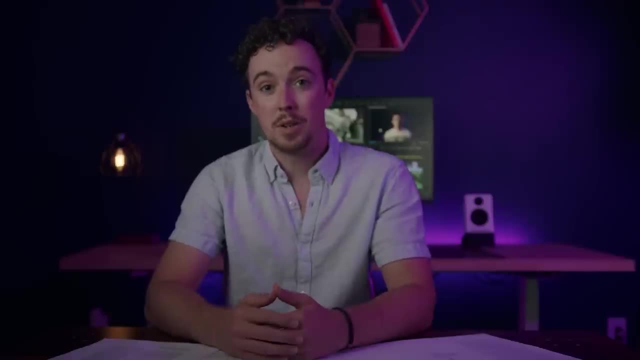 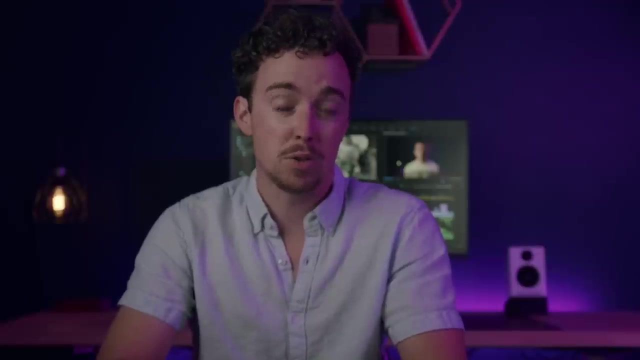 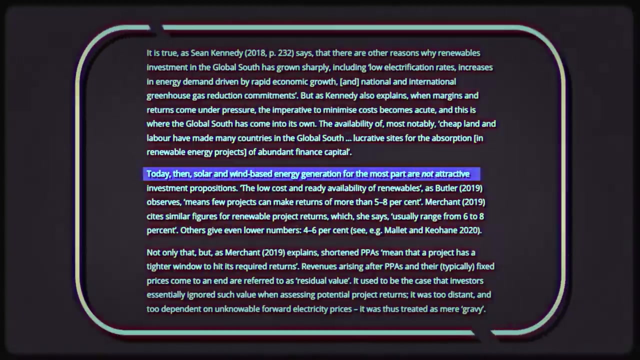 return on investment, And the sad part is that that just won't happen, and they already know that, According to just about every estimate, no one can expect those kinds of returns on renewables. Quote Today, then solar and wind-based energy generation, for the most part, are not attractive investment. propositions. The low cost and ready availability of renewables, as Butler observes, means few projects can make returns of more than 5-8%. Merchants cite similar figures for renewable project returns, which she says usually range from 6-8%. 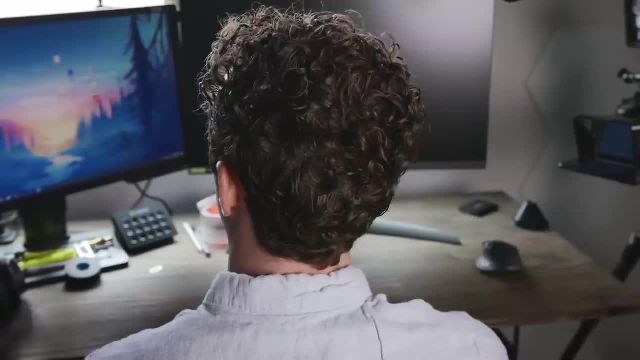 Others give even lower numbers: 4-6%. Shell, on the other hand, says that the cost of renewables is much lower than the cost of solar and wind-based energy generation. They say Well, BP, Total and all their little dinosaur-juice friends can bask in the great press of being. 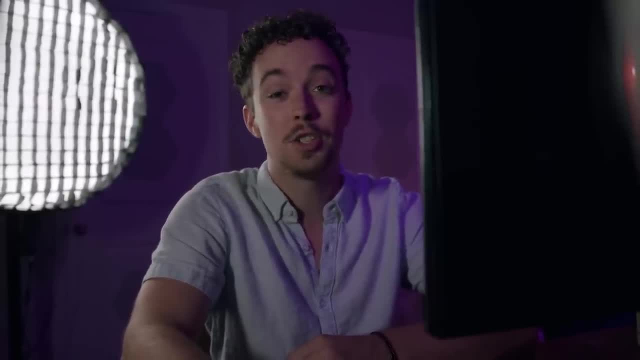 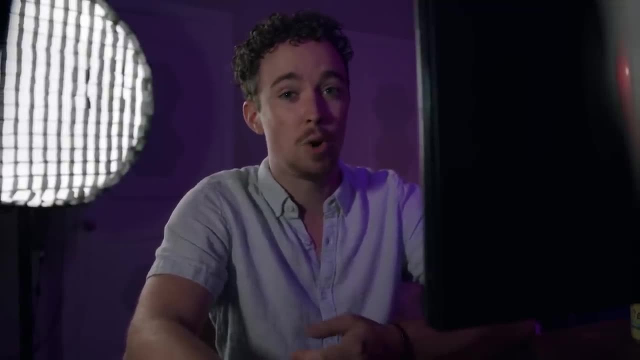 the good fossil fuel companies committed to righting their wrongs and transitioning us away from fossil fuels. But behind the scenes they know they'll never fulfill their arbitrary profit conditions and therefore they'll never need to keep their promise. They will not invest in renewables and they have an out. 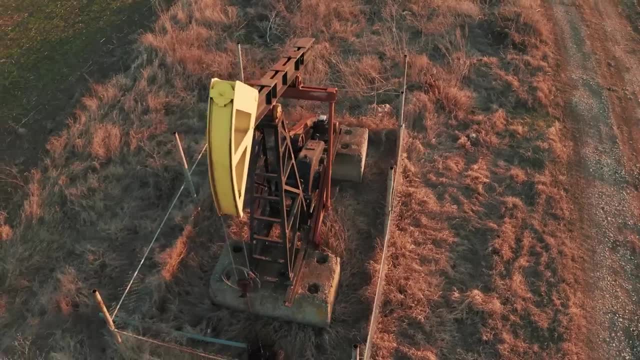 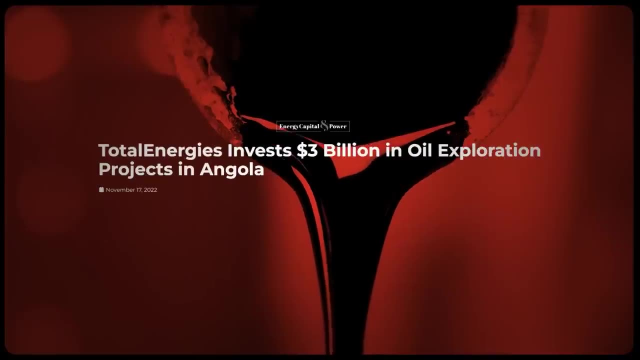 Because, by contrast, oil and gas are still massively profitable. At the same time these net zero declarations were being made, Total was opening up no way, and they had no chance of winning. Shell, too, had 21 new projects announced all over the world, and BP successfully added. 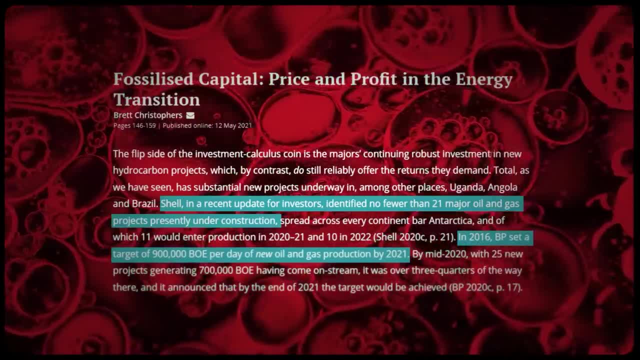 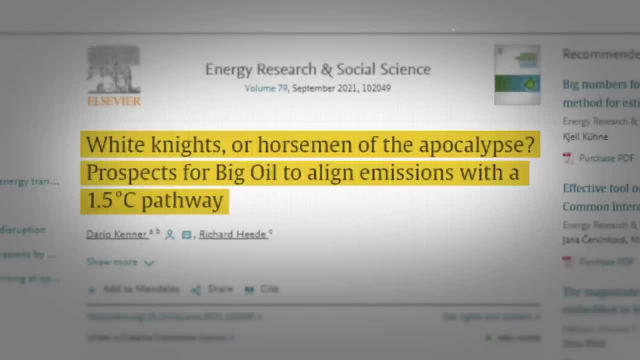 900,000 barrels of new oil and gas production a day between 2016 and 2021.. Compare that to renewables Between 2010 and mid-2018,. BP only allocated 2.3% on low-carbon investment, Shell 1.3%. Chevron 0.23% and ExxonMobil 0.22%. That's a lot. They are not spending their money on renewables. Actually, that's not true. A big chunk of these tiny investments actually went toward solar farms and windmills, which 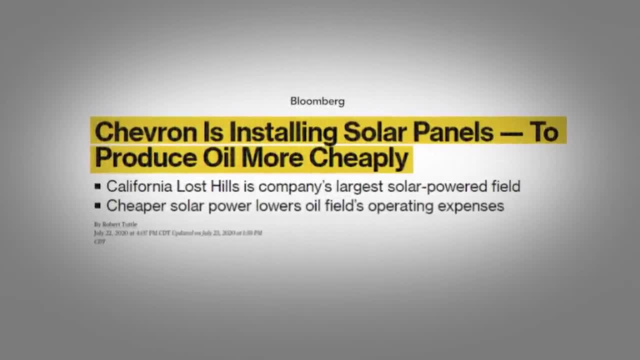 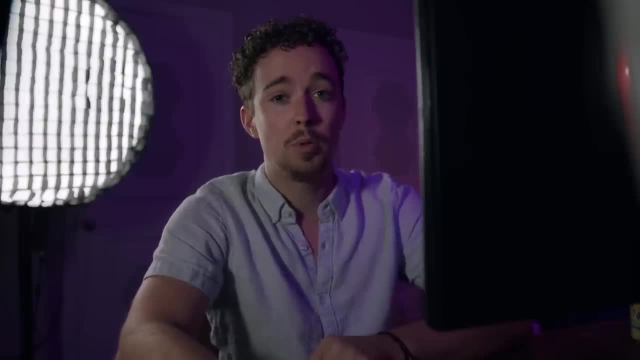 were used exclusively to power new oil fields. so there's always that. And fossil fuel companies aren't the only ones playing this game. BlackRock, Vanguard and State Street are commonly referred to as the big three in asset management. Like fossil giants, they've made the same commitments: to be more sustainable. 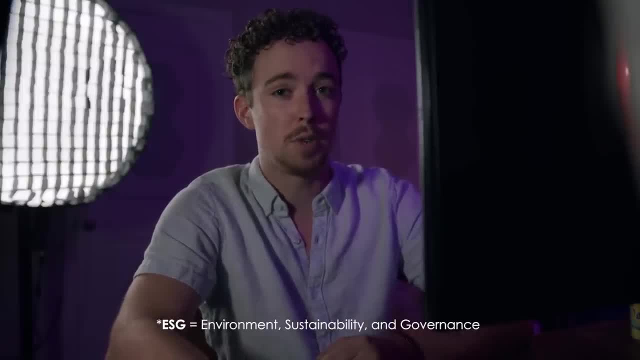 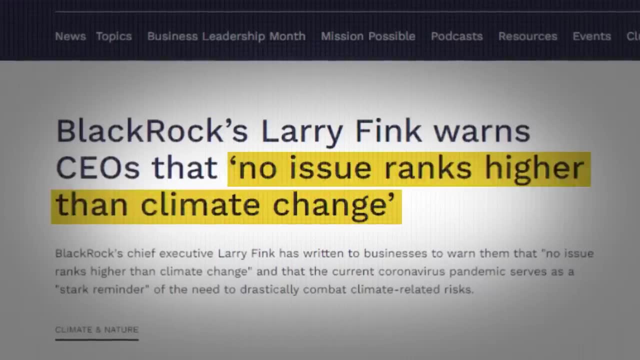 They've introduced ESG funds And they said their requirements for these funds would become more robust in keeping with the urgency of global warming. BlackRock CEO Larry Fink has even gone out and said that quote: no issue ranks higher than climate change. Given that together, these three companies have north of $20 trillion in assets, control 20% of shares in the average S&P 500, and have- quote- the highest CO2 emissions from holdings in fossil fuel companies, their actions could have a huge impact on hundreds of thousands. 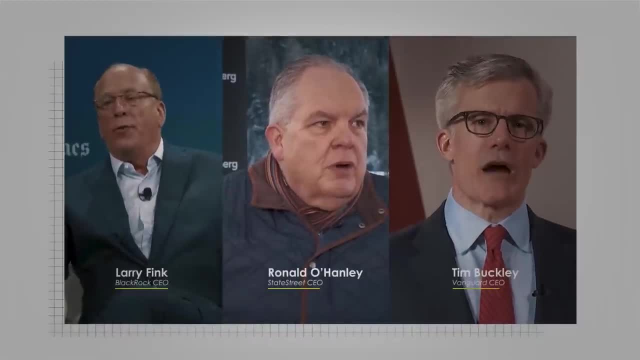 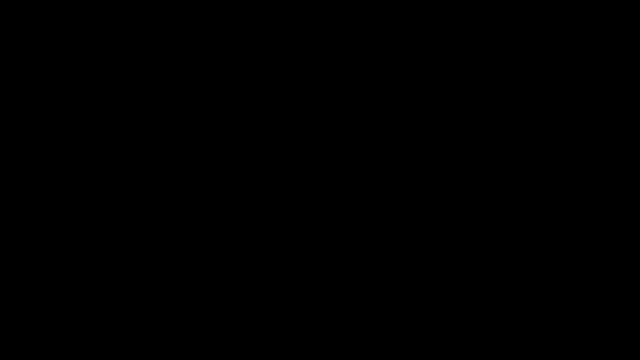 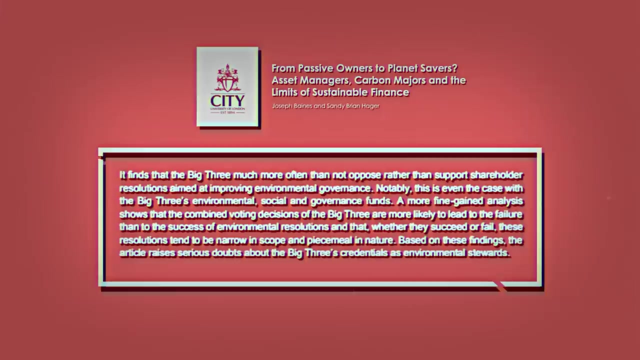 of companies and the environment. That's a big deal. They have the wealth and massive corporate ownership to push companies across multiple high-carbon industries toward sustainability. So what do they do, Not that A 2022 study of the actions of the big three asset management firms found that quote? 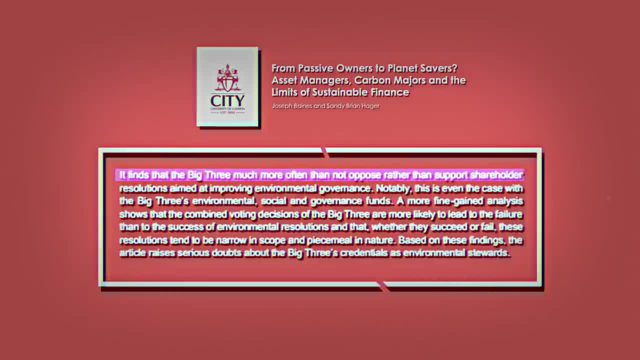 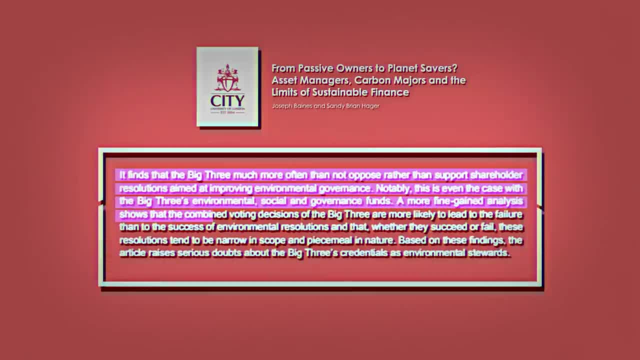 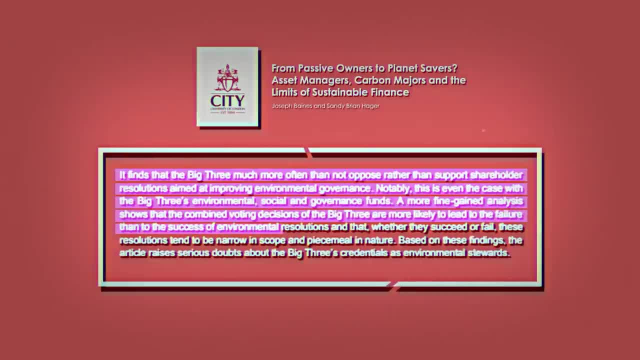 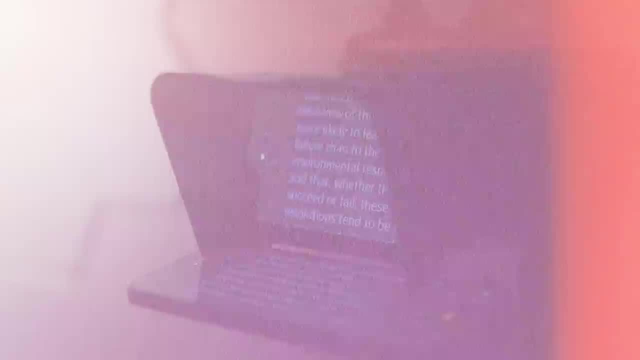 are more likely to lead to the failure than to the success of environmental resolutions and that, whether they succeed or fail, these resolutions tend to be narrow in scope and piecemeal in nature. To summarize this whole chapter: fossil fuel companies and massive firms that control entire. 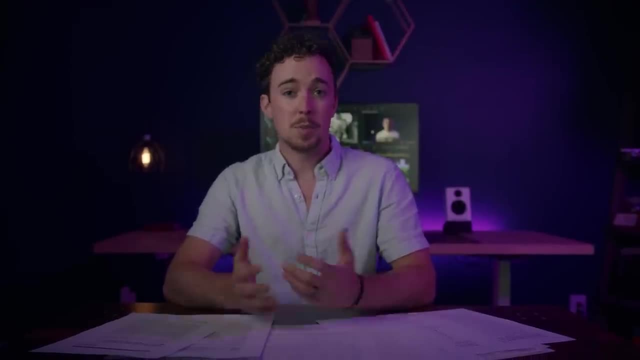 chunks of the economy do not care about sustainability. As much as they may send out press releases or get quoted in major news outlets for saying they think the earth is good. they're not. As much as they may send out press releases or get quoted in major news outlets for saying 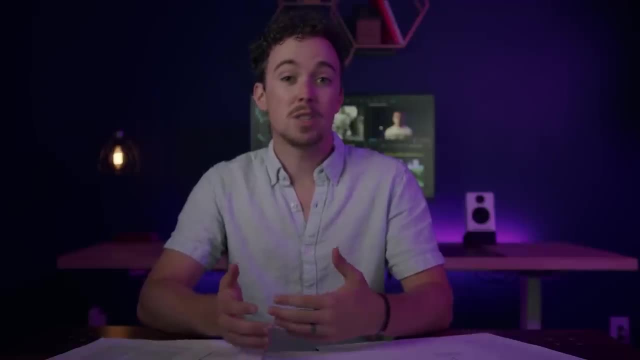 they think the earth is good. they're not. They are guided by one thing: only—profit. It's not just greenwashing, It's not just like bad CEOs who need to be swapped out with nice CEOs. It's what the greater economic system demands. It's what the greater economic system demands. Under capitalism, production is always initiated on the basis of prospective profit. Unlike what liberal economists might tell you, it's profit—not price—that matters to our economy, To built-in tax and finance mechanisms—they're not here to buy electric cars, etc. 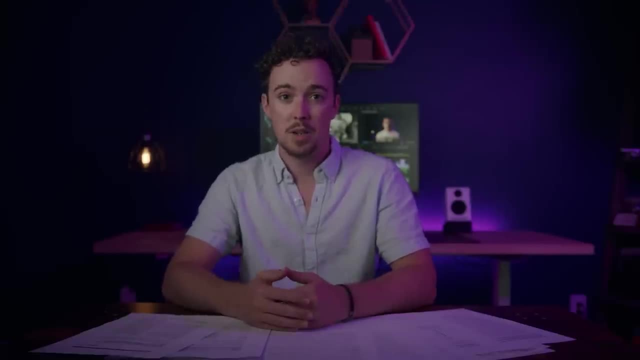 To built-in tax and finance mechanisms—they're not here to buy electric cars, etc. It's a place to gather that money Entering conflictman orперies is only tough Entreping problems or being messed up because they aren't wildly type deep outlet points and 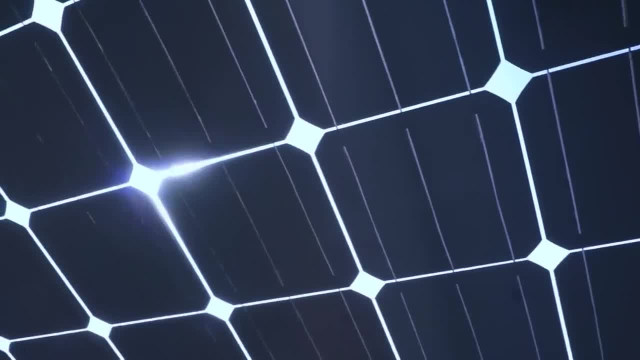 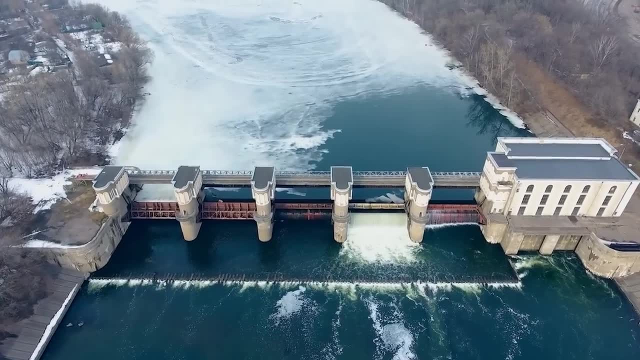 come with the promise of change. Cheaper prices are good for consumers, but a good is only worth producing if the margins are also good for the seller. And in the world of renewables, the International Renewable Agency found in 2018 that quote. 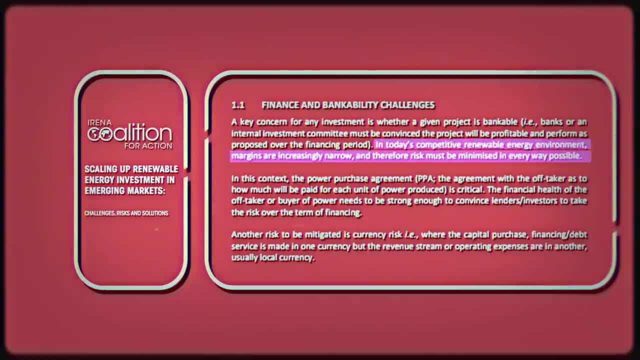 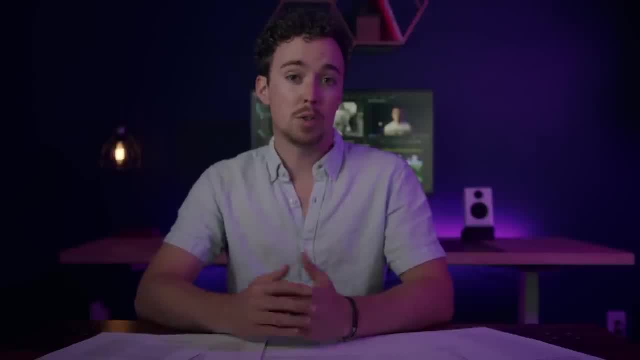 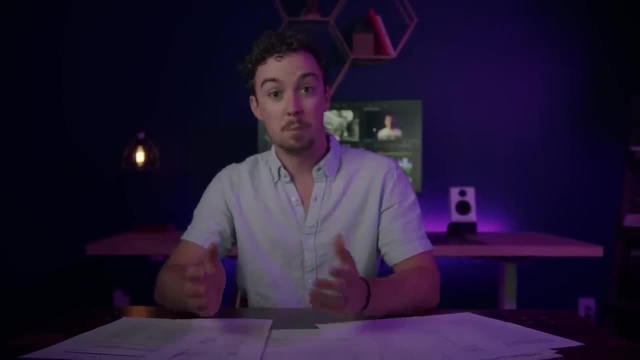 the margins are increasingly narrow. There's just no money to be made in renewables and that's enough for investment and deployment to stall. More than any of the other qualms we might have with solar, it turns out this completely arbitrary limitation, the ability for a few to enrich themselves in the transition process. 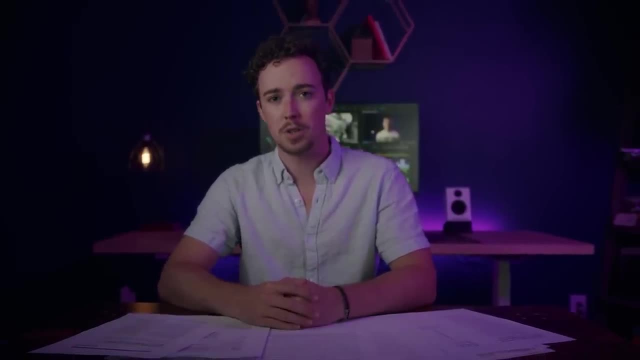 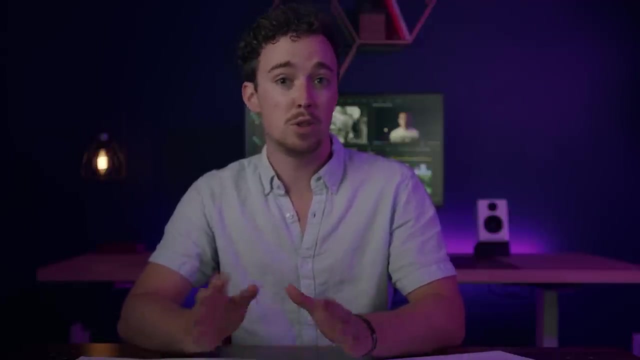 may actually be the biggest roadblock to a more sustainable energy production system. It's not enough that we need to release fewer greenhouse gases in the atmosphere. It's not enough that it's now cheaper and easier than ever to do so. It will not happen unless someone finds a way to make money off it. 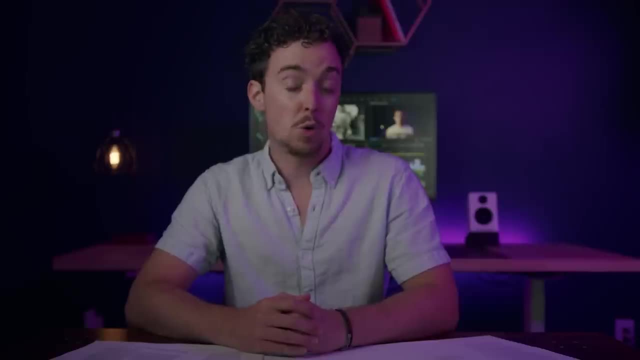 And that's just sad. And do you want to know how I know this transition won't happen? just because of cheap solar prices, Beyond all the evidence I just cited of what companies are doing right now to make money. now, the reason the transition to renewables isn't happening is because of one incredibly 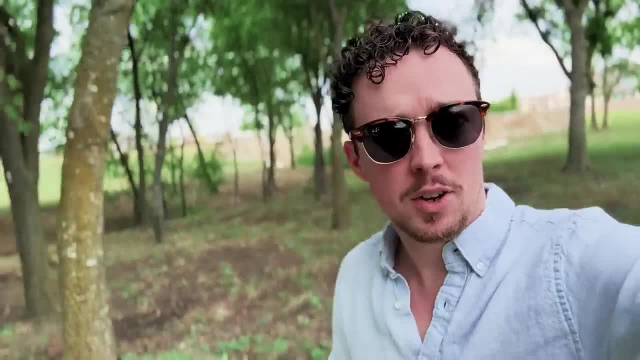 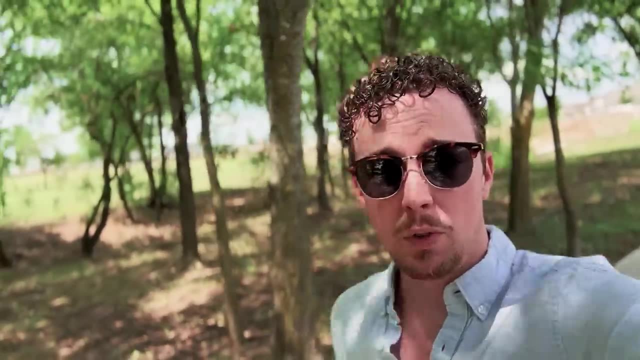 simple word: Exploitation. Okay, folks, we are going on a detour. I'm about to summarize this book way too quickly. To understand our predicament with transitioning from fossil fuels to renewables, we can look at how we transitioned power sources during the Industrial Revolution. 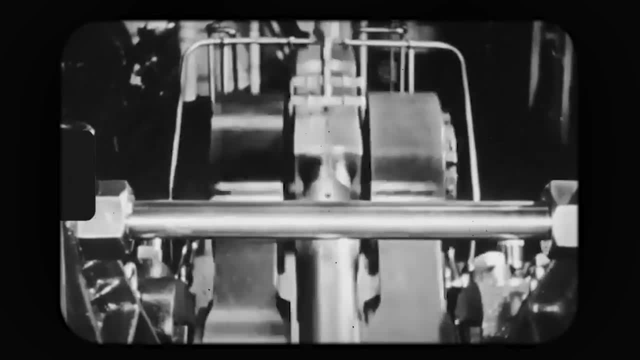 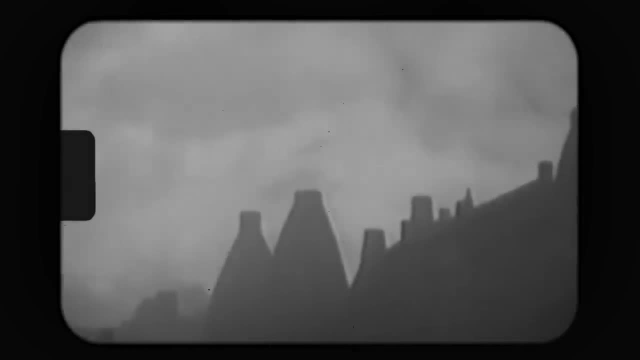 Back then we went from water power to steam power, meaning we started using fossil fuel combustion to power stuff. While flowing water and fossil fuels each had their own advantages, the main one for fossil fuel power was that you can use it to make a box of fire, and it'll make a 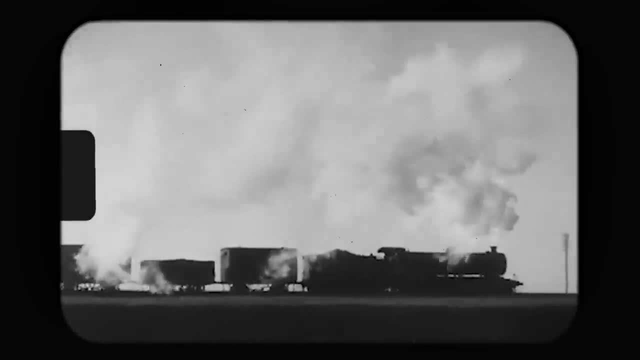 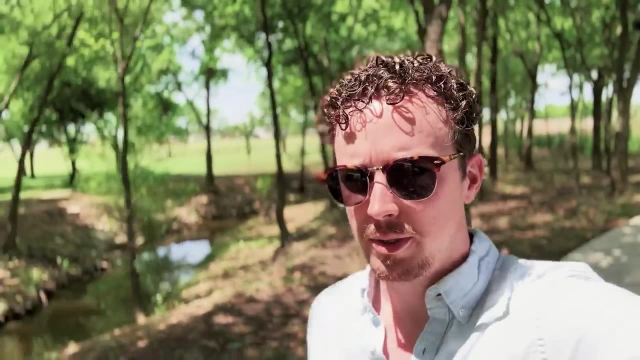 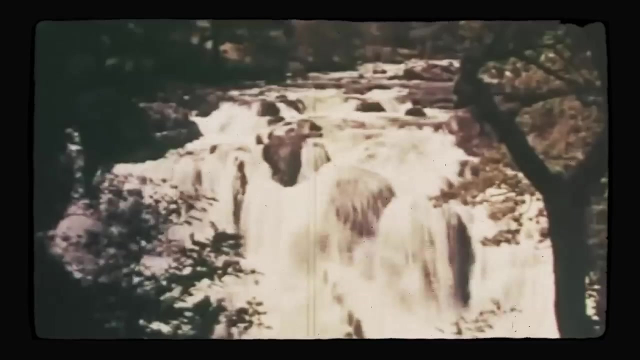 train move, But that's about it. In the competition of who was going to power factories, water and coal were equivalent options, Except that water was cheaper. Unlike coal, water takes very little human labor to extract energy from, And, given that it could produce as much power as steam that waterfalls were abundant and 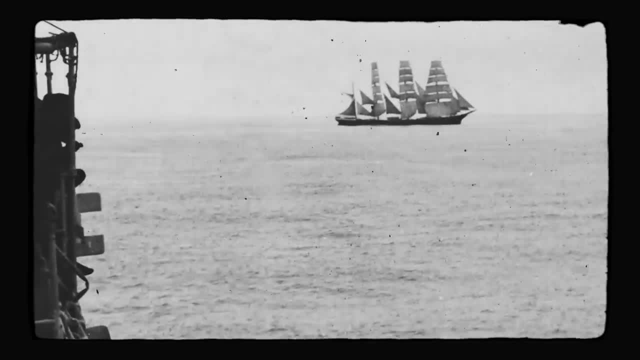 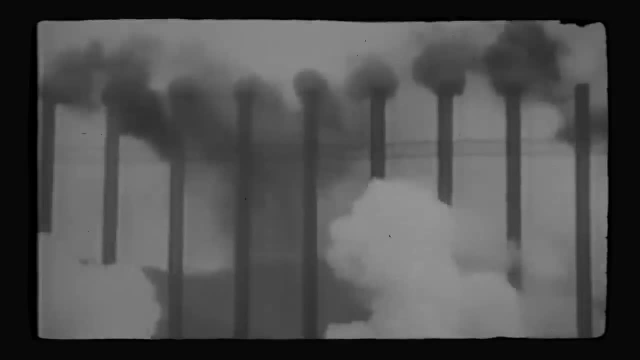 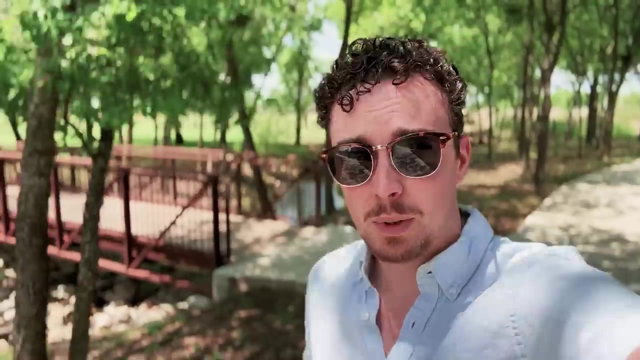 that it was cheaper. if we are to trust liberal economists, history should be the same. We should be able to make a difference. The theory should be that steam, and therefore fossil fuels, would only have limited applications in things like transportation, But overall water should have dominated industrial production. 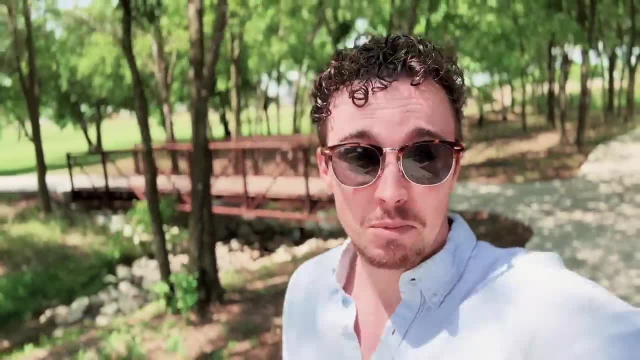 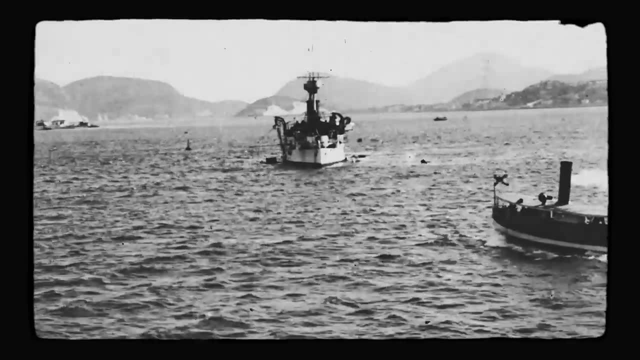 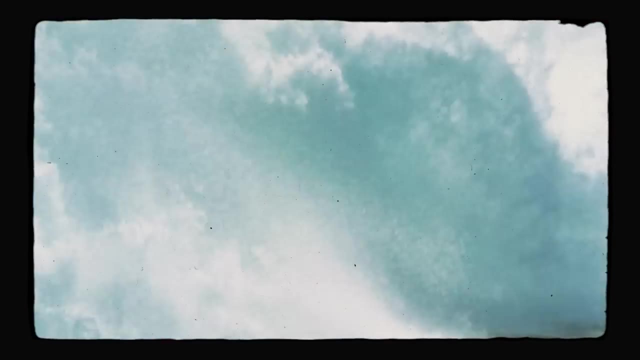 But that's not what happened, because right after I finished saying that sentence, cities all over Britain started filling up with black smoke. My bad, That's because the thing that differentiated steam and water was that steam was better for exploiting humans And therefore, although water was a cheaper source of energy, it was a less profitable. 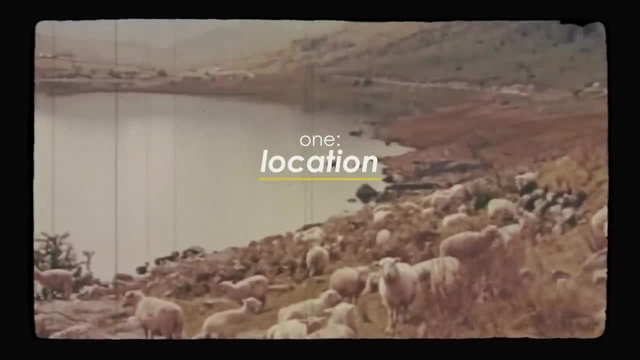 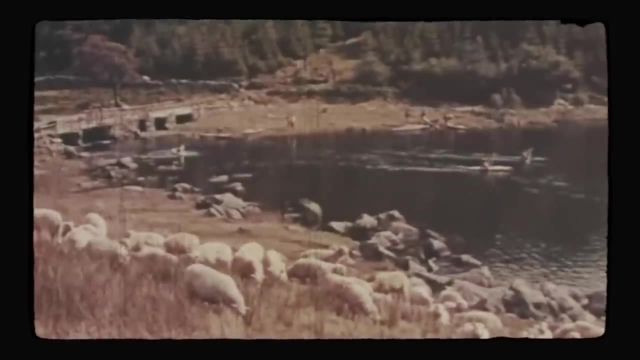 one One. flowing water sources are pretty often out in the countryside. If you want to use them, you often need to bring people to the water, And if those people you moved closer to the water strike, it's hard to find scabs to. 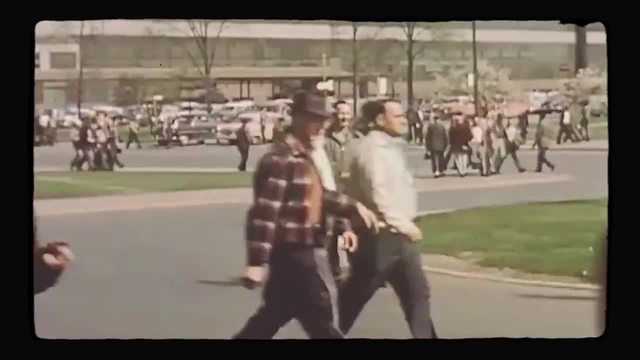 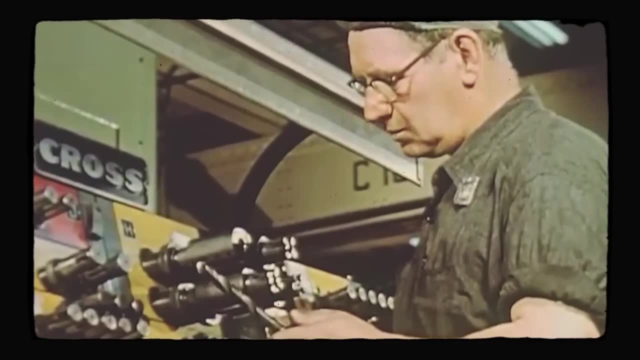 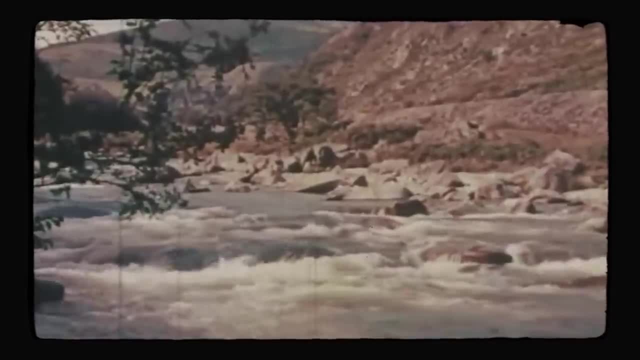 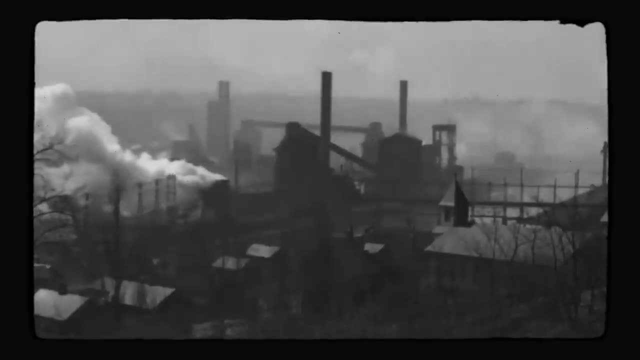 And that's why we're here. And that's why we're here. Two: water has its own rhythm. Sometimes it doesn't flow and therefore people don't work In the city, though as long as you keep shoveling coal, you can work through the night every. 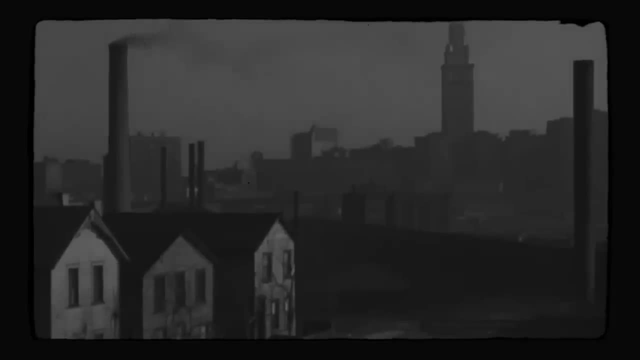 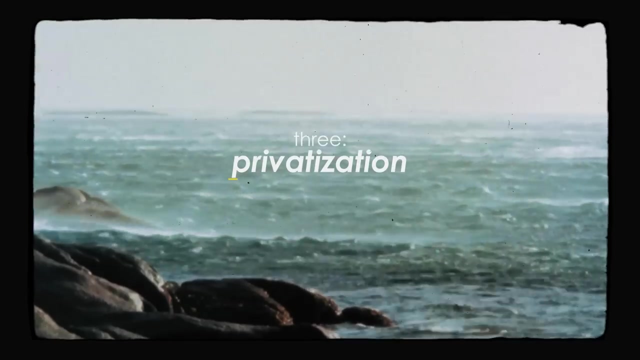 day of the week. for as long as you can get people to stay in the factory. The only limit on exploitation is the amount of people and the amount of coal, And there was plenty of both. Lastly, water is hard to collect and privatize. 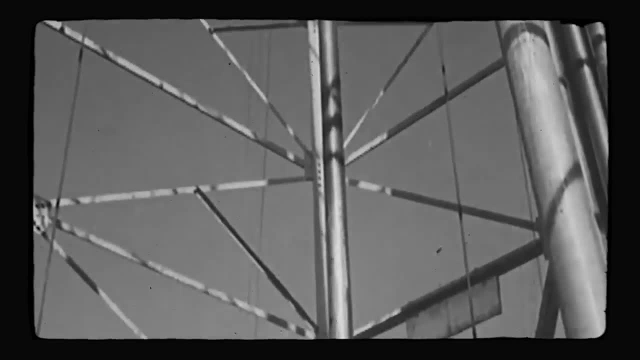 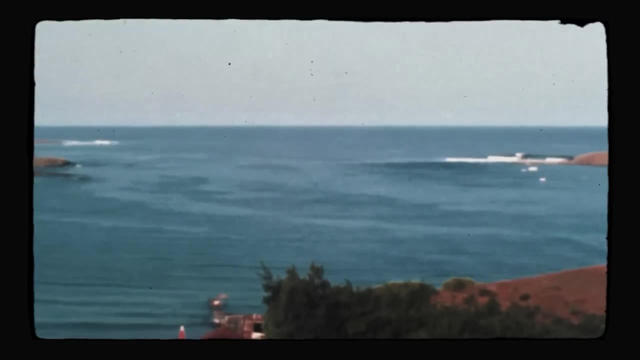 A coal mine or an oil well is fundamentally just a hole in the ground surrounded by guns. It's easy to claim as your own and to enforce that claim with violence in a way. that is much harder with a naturally occurring water source that can run for miles. 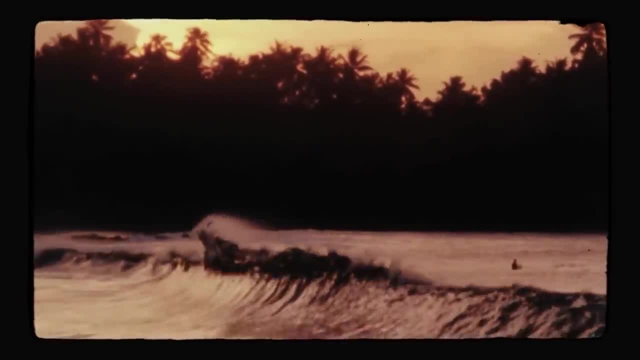 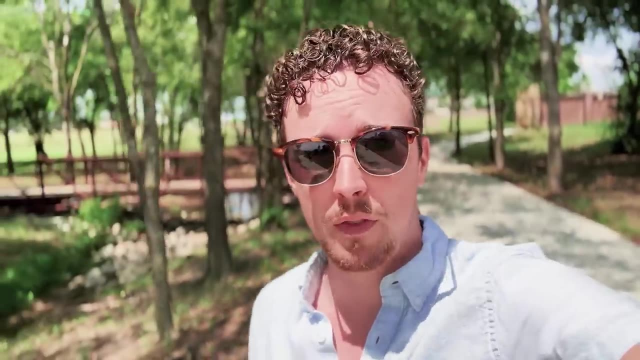 And if you're thinking about building a reservoir, well, that gets a little too community project-y for privatization. All together, this meant that even though water was cheaper, it was less profitable as a source of energy. Fossil fuels- coal, specifically- was fantastic for the burgeoning capitalist class. not because 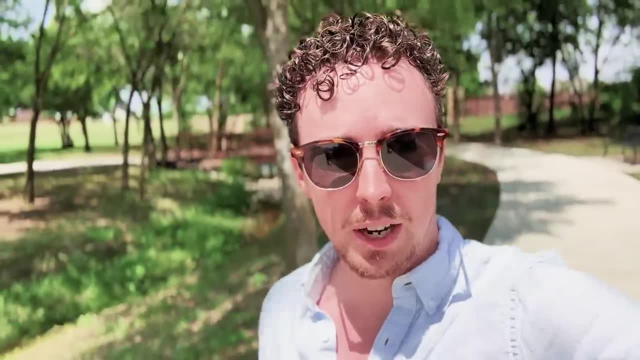 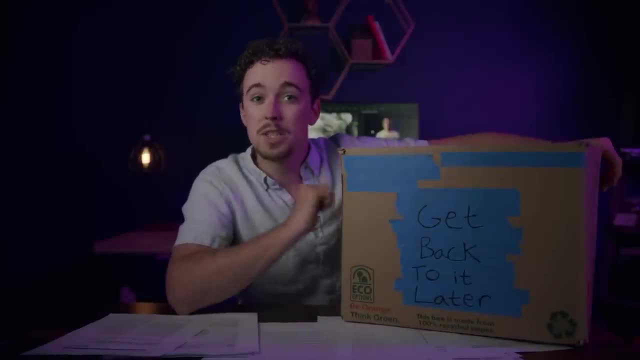 they were cheaper, but because they were an excellent source of surplus value. Okay, detour over See. I told you we'd come back to this. The reason I took that massive detour is not only that, it reiterates this video's main. 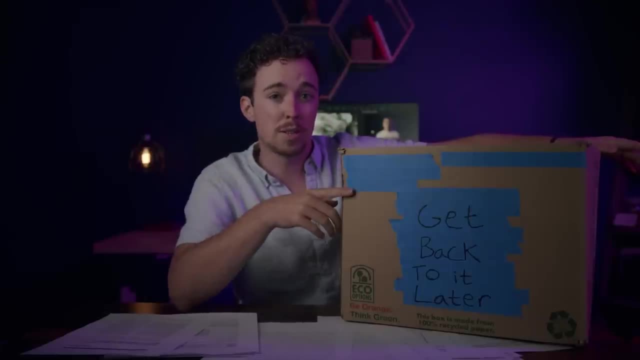 point, which is that under capitalism, profit matters, not price, but it's actually also giving us a bit of insight into what's happening with renewables right now. In this video, you've heard me say over and over again that renewables aren't profitable. 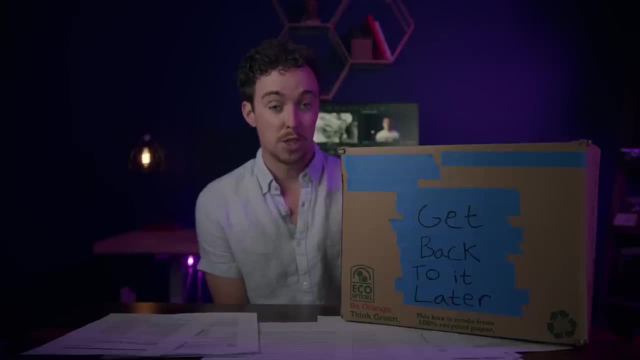 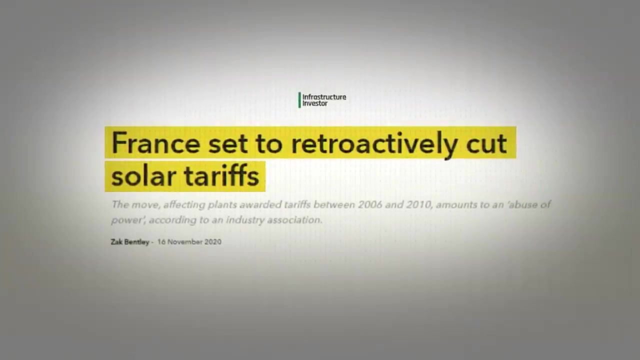 and that's not exactly true Saying renewable energy isn't profitable, Since governments have slowly stopped guaranteeing high prices to renewable energy providers – something you won't be surprised to find out that the fossil fuel industry lobbies for – the efficiency race, which is good for all of us, has been bad for those trying. 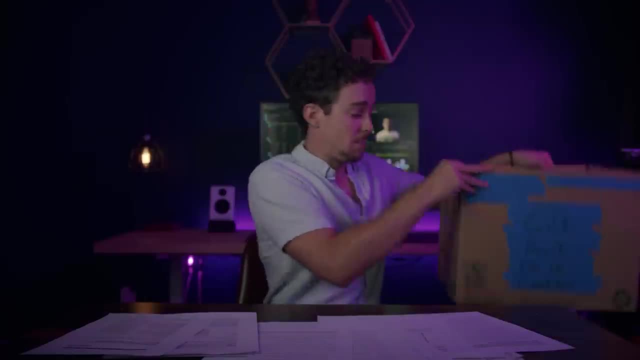 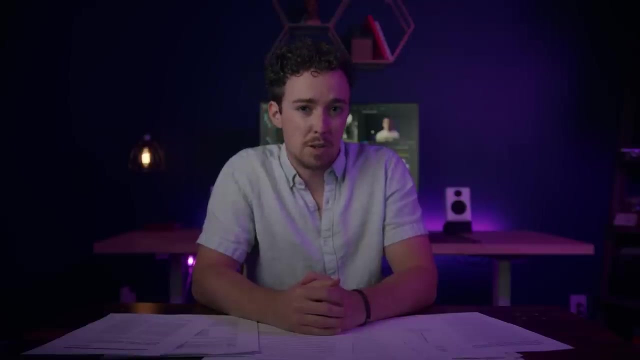 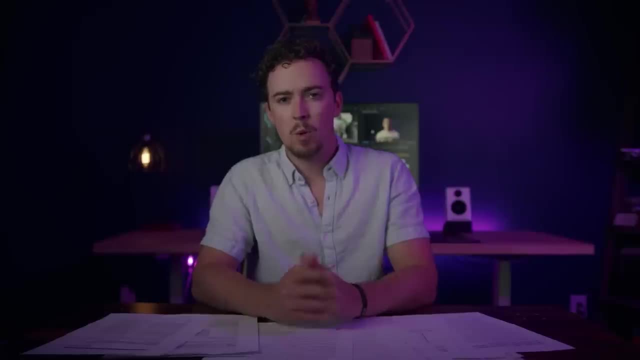 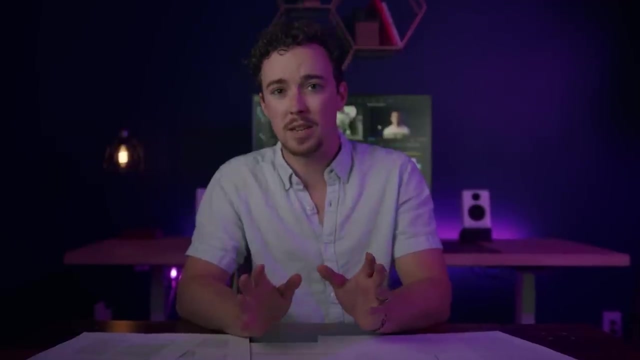 But it doesn't stay the same, but needs a lot more guns. So where's the money going? All these places keep divesting from fossil fuels. there was investment in renewables, even if it is stagnating, and ESG funds seem to do well. So where is that? The truth is that money goes to the parts of the process where exploitation is still rampant and guaranteed, Basically manufacturing solar technology and extracting rare earth minerals from the ground in countries in the periphery. This is basically a market store of materials. 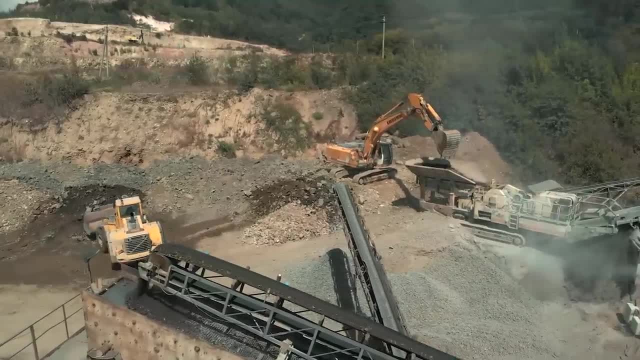 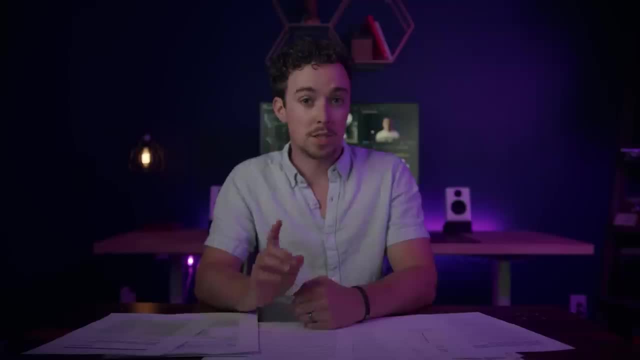 The parts of the solar business that are still incredibly ugly to look at, because they are either rife with violence or places where pollution isn't a cost companies need to worry about. That's where privatization is easy, where labor is cheap and where the margins are. 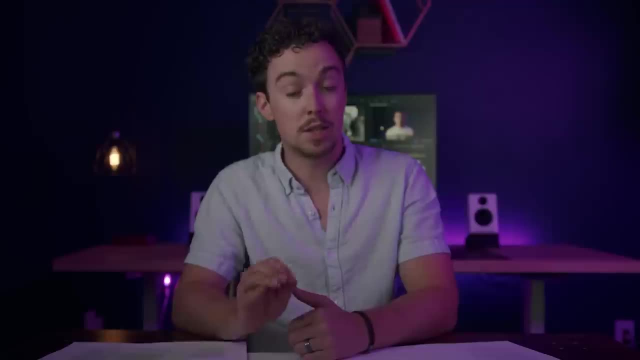 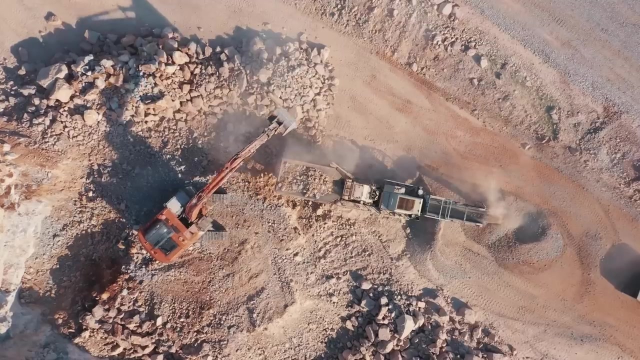 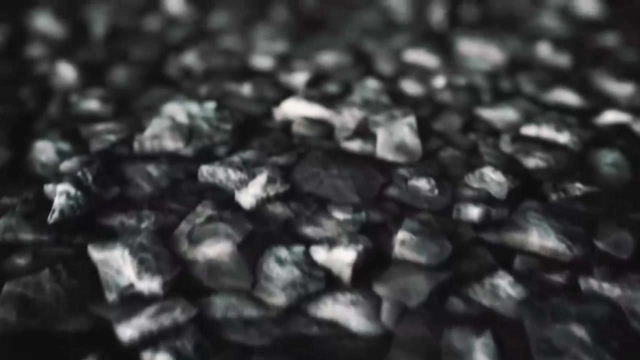 therefore still high Where exploitation is still possible. That's where the money goes, And before this seems like another path to the same solution: a less carbon intensive economy. nothing about this ugliness is intrinsic to solar Mining. these resources doesn't need to be violent like it is or nearly as polluting. 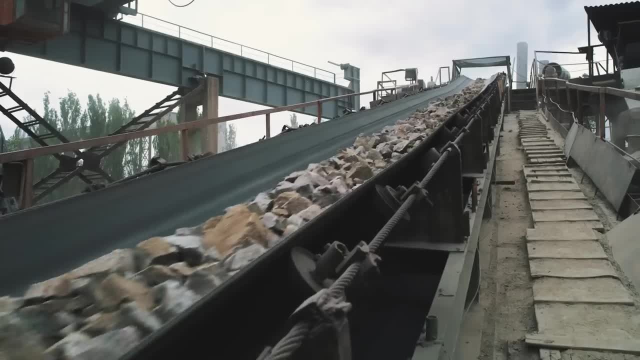 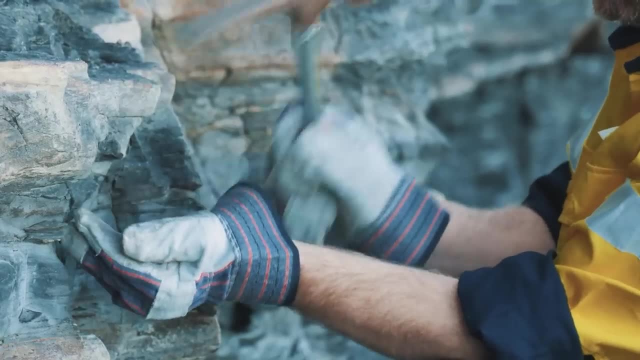 or need to happen on such a large scale. If we simply allocate energy effectively and break the requirement of constant, unending economic growth, we'll need way less of this stuff. If workers weren't so disempowered, they wouldn't have to accept these awful conditions. that produce such great profit margins. If democratic bodies could enforce environmental stewardship norms, the quick and dirty pollution of the mining process could be kept under control. It is only when growth and exploitation, and therefore profit, is a requirement for sustainable action that this ugliness sticks around. And it is only because it is there and hasn't been purged by collective social action that capitalists make a profit. Bottom line solar and renewable energy generally will probably need to be a part of how we limit the worst of climate change. 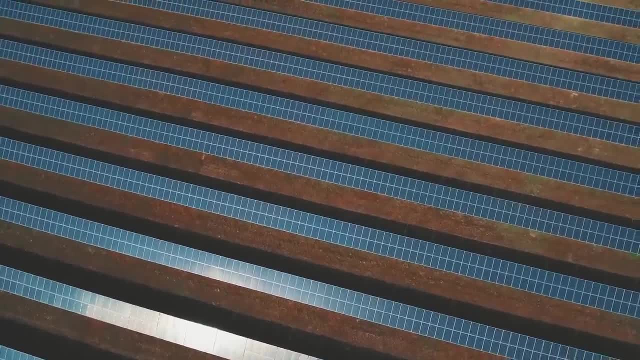 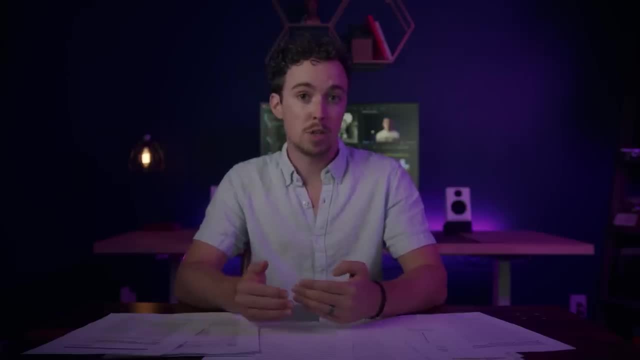 But so long as moving in this direction requires us to find profit in the process, it will continue to come with massive drawbacks. It will place the burden of remaining on the ground. It will place the burden of remaining within our planetary boundaries on the most exploited. 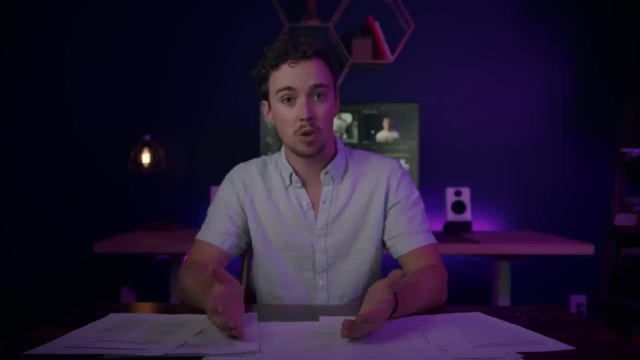 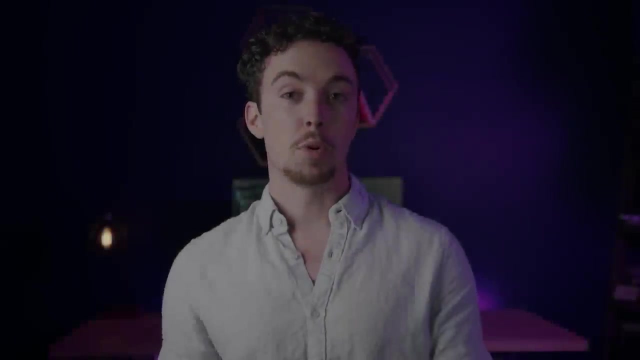 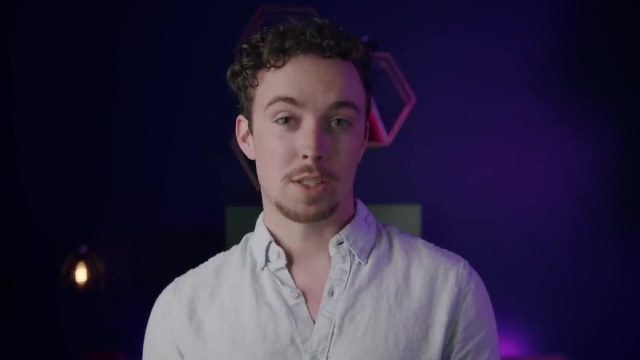 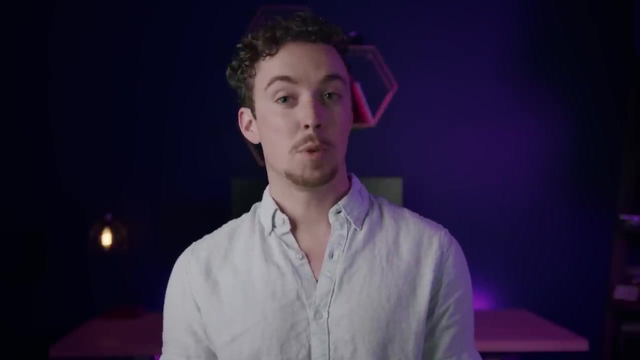 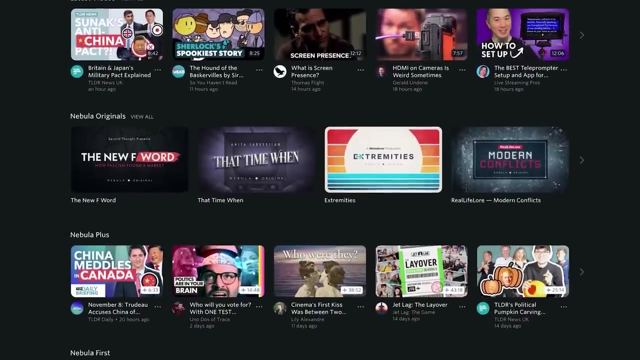 people in the world And will not come soon enough to save us all, Only the most fortunate. That is unacceptable. There is no capitalist path to climate justice. There is only one: including us. The replacement of climate justice in this era is half the game. 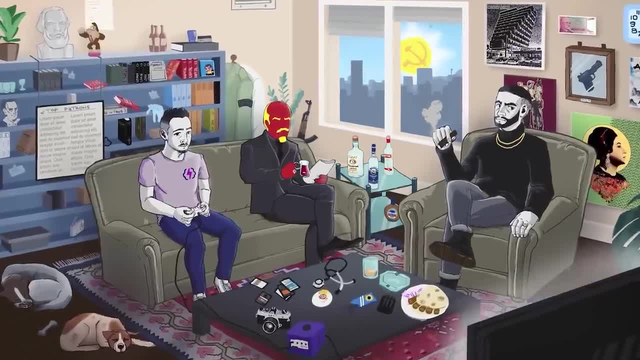 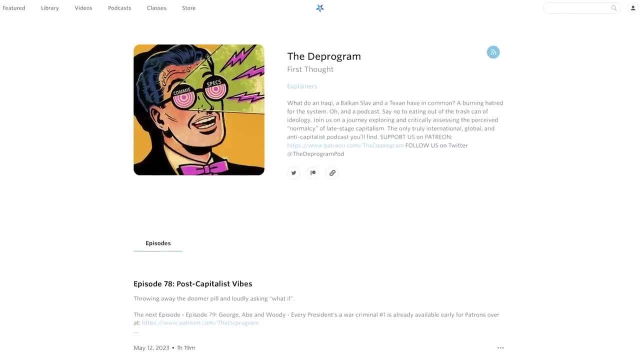 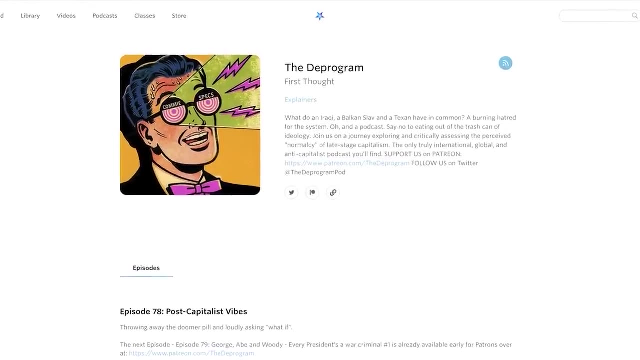 The기로. Mr President of the RepublicENEEEEEEE I on the I N E o V S, I S S S our words carefully to avoid age restriction or demonetization. And now, if you sign up with MyLink, you'll also get access to the new Nebula classes. 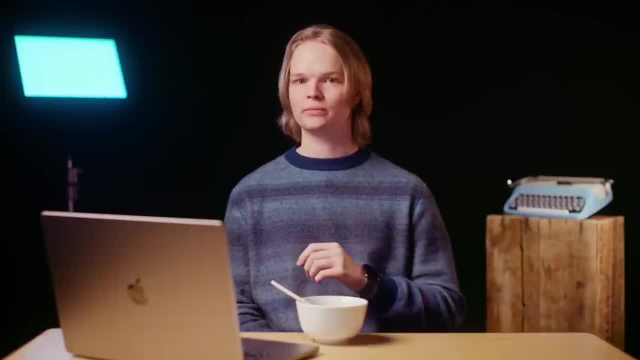 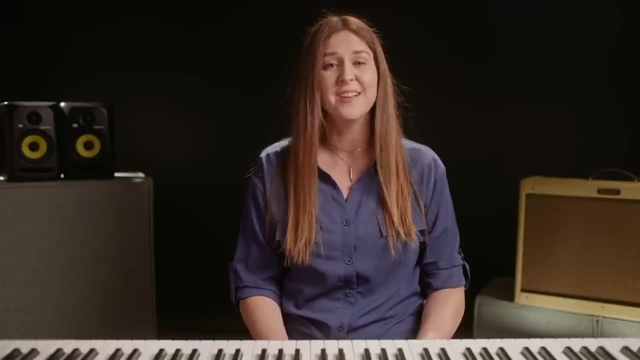 where creators host classes on how to be a creator. There's something for everyone, and it's another way for you to take a peek behind the scenes and see what really goes into making content: Your favorite creators teaching you how to create. In my opinion, that's pretty cool.